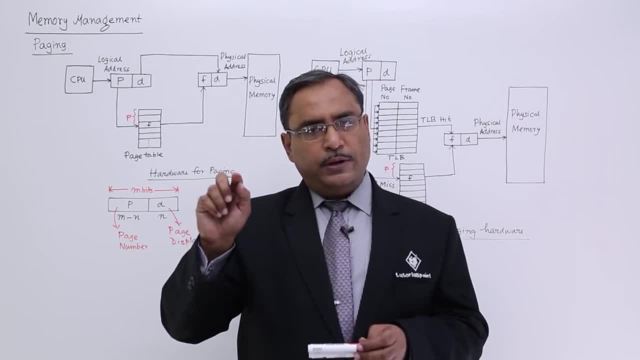 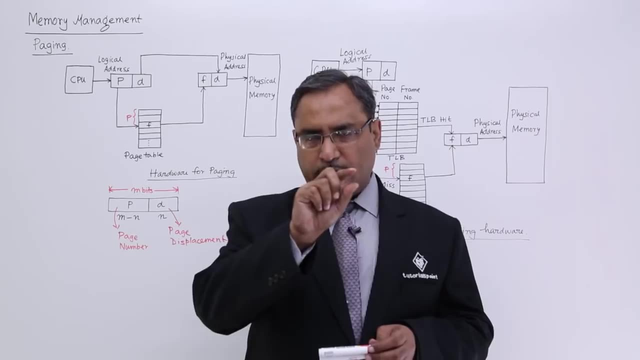 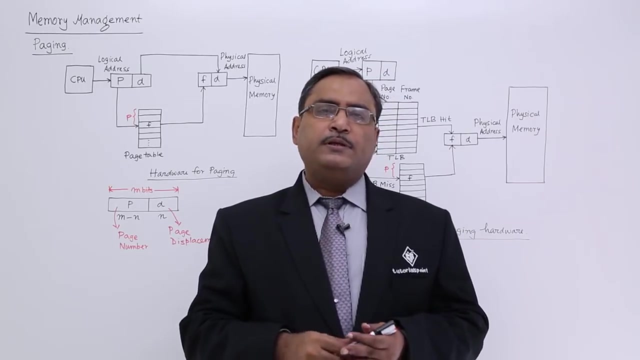 equal sized partitions, partitions, and each and every partition will be known as a page, and the physical memory space will be divided into equal such partitions and they will be known as a frame. Page size is equal to the frame size. That means, whatever the size of the page, accordingly the frame 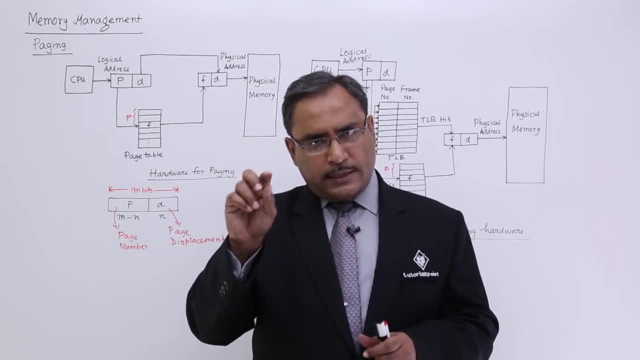 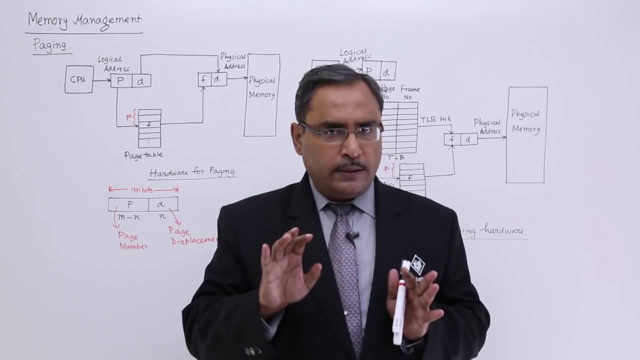 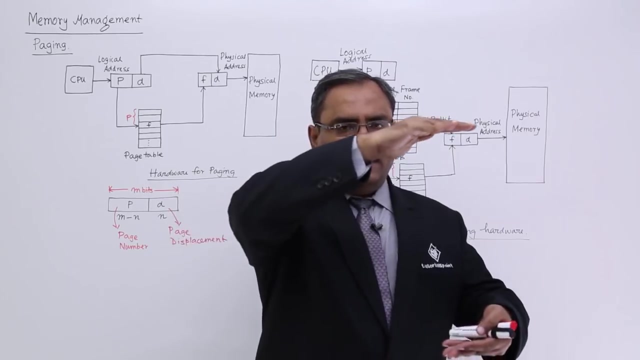 size will be decided. So whenever a particular page is getting loaded to a certain frame, then I should think that there will be no free space remaining. So that is the main concept. So the program space will be known as the logical address space and the physical memory. 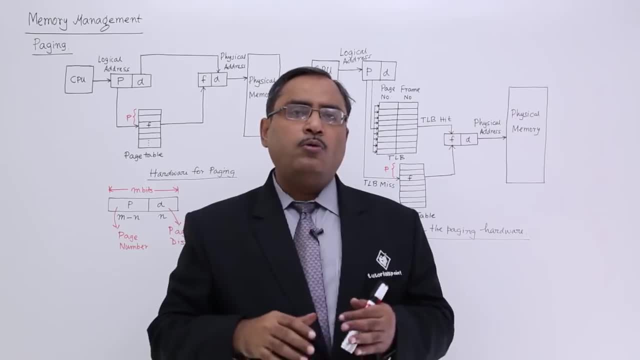 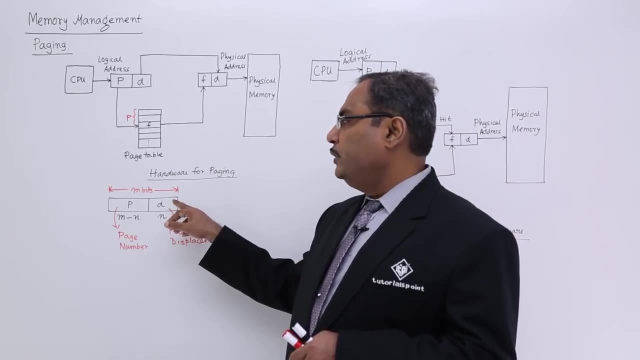 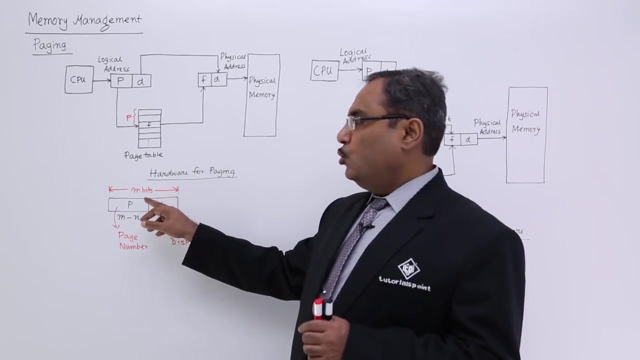 space will be having the physical address space. Now how does it take place? Let us suppose we are having one page with the m bits. We are having one memory address with the m bits of These m bits of memory address will be divided into two parts. One is the p and the one for the d. Let us suppose d is having 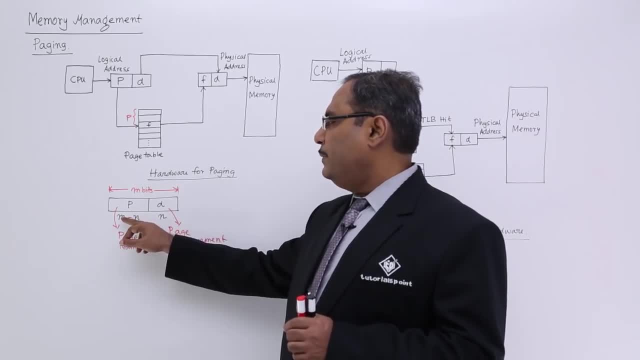 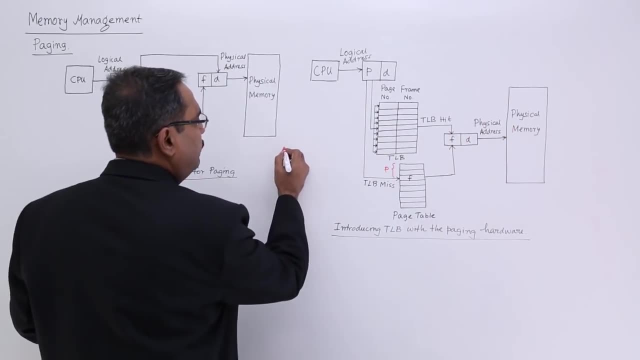 n number of bits, So remaining p will be having m minus n number of bits. I think that problem is not clear. Let us suppose there is a particular space of 4096 bytes, So obviously to address this particular space I require 12 bits. I required 12 bits why? Because 2 to the power. 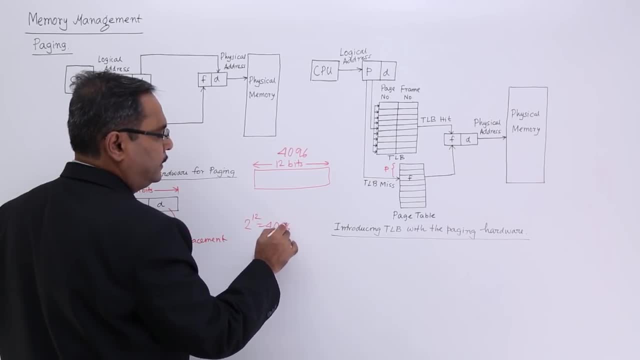 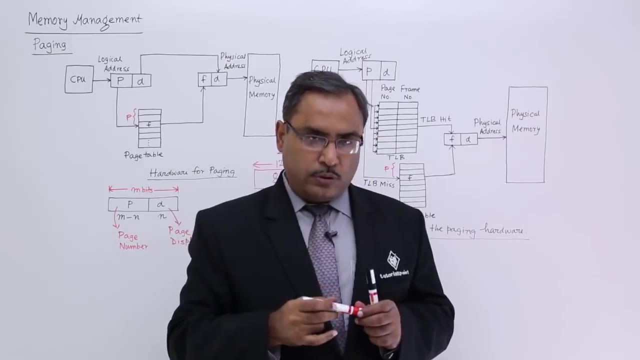 of 12 is equal to 4096.. Out of those 12 bits, I am dividing it into 8 plus 4, I am dividing it into 8 plus 4.. That means the displacement will be of 4 bits and the page number will. 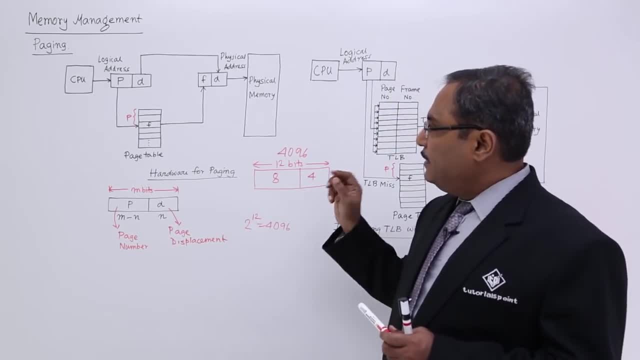 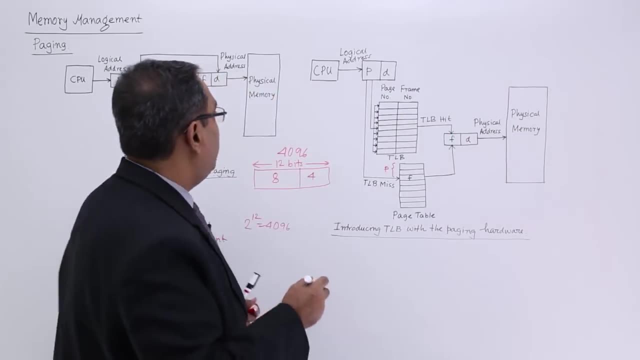 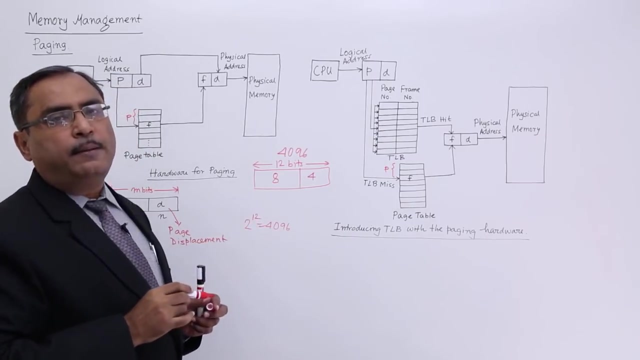 be of 8 bits. That means each and every page will be having 16 locations, because 4 bits can have 16 locations. That means what is happening: each and every page will be having 16 locations and in this way, we will be having 256 number of pages because 2 to the power. 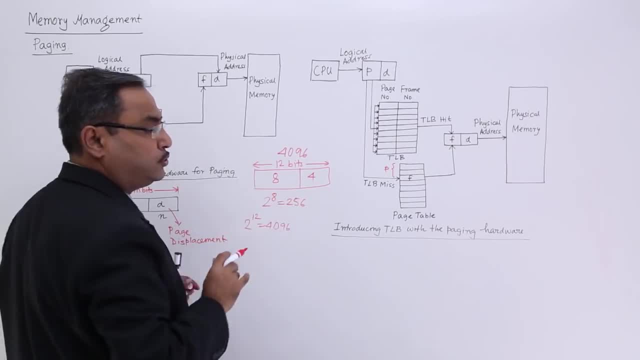 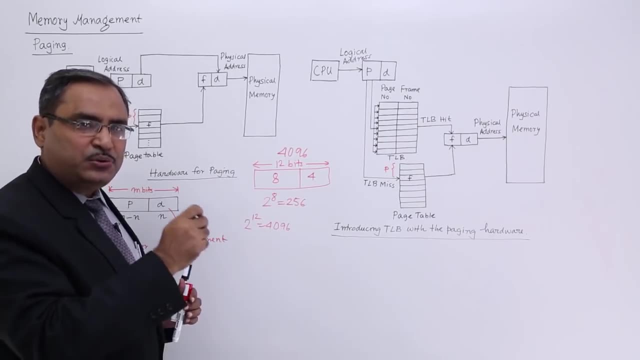 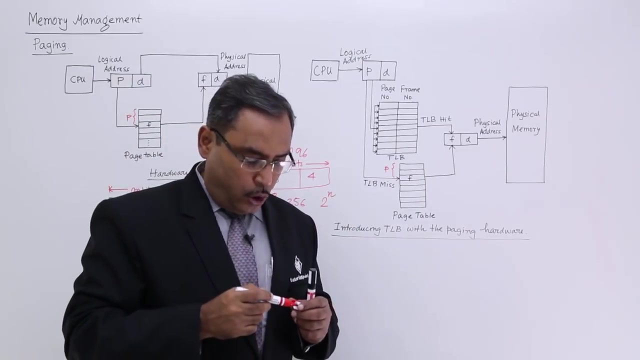 of 8 is equal to 256.. So that will happen. That is why one favorite question is there always. the question is there: why the page size is always of the order of 2 to the power of n, Why the page size is always of the order of 2 to the power of n? Because the answer.